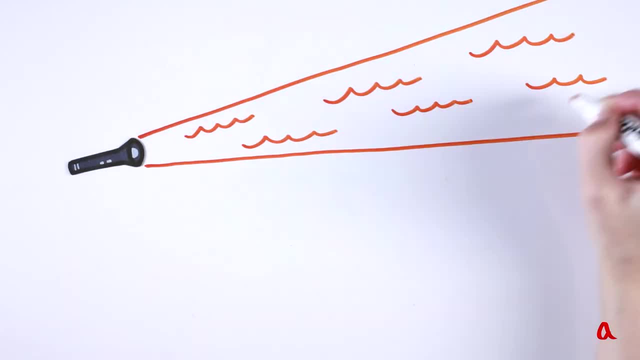 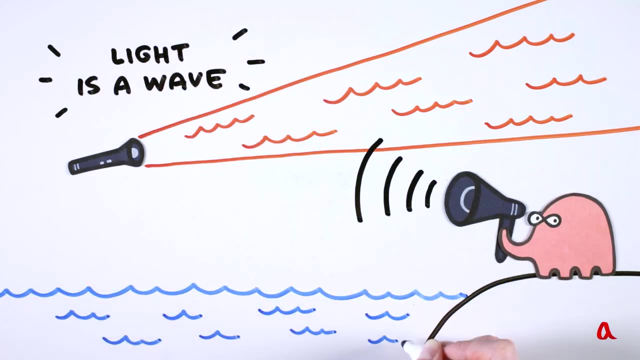 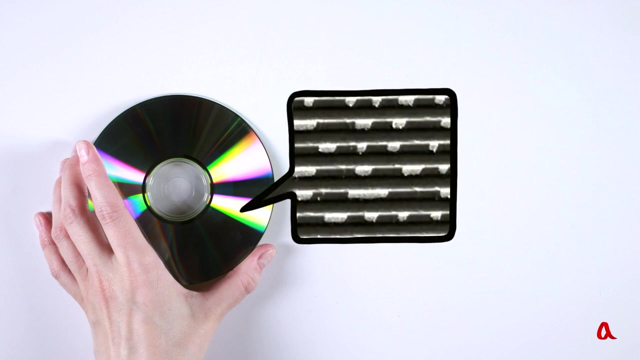 All further explanation is based on the fact that light is a wave And light waves in a sense behave in the same way as sound waves or water waves. Now let's talk about how a CD works. Its surface is marked with parallel tracks, the distance between which is only 1.5 microns. 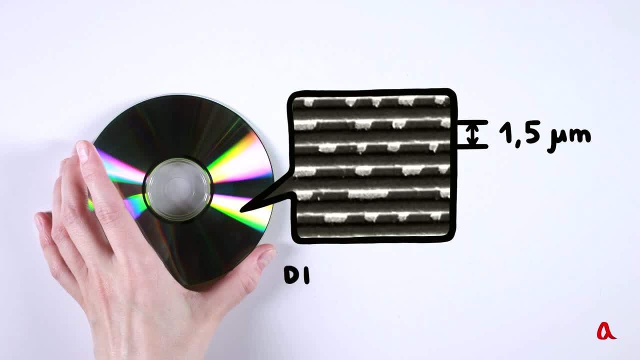 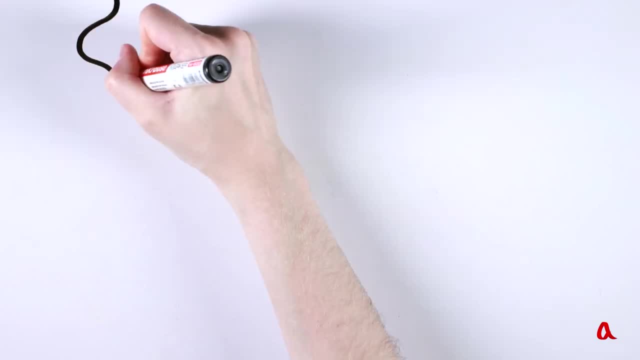 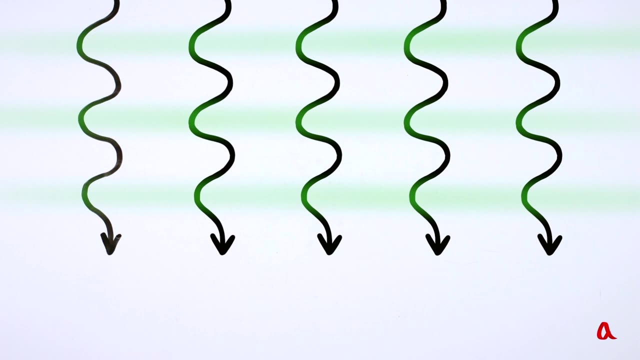 In optics, such a device with parallel strokes is called a diffraction grating, and the step between the strokes is the grating period. Let the light, with a certain wavelength, fall onto the surface of the disc at a right angle, just like a wave rolls onto the shore. 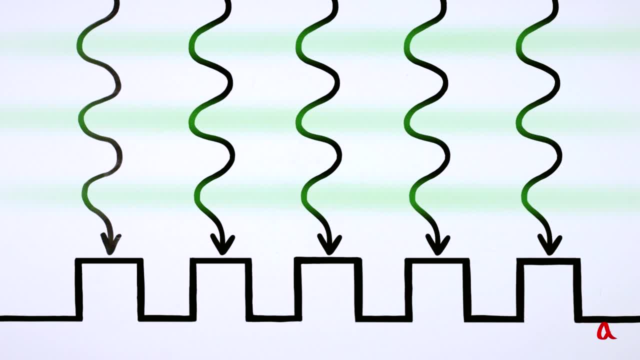 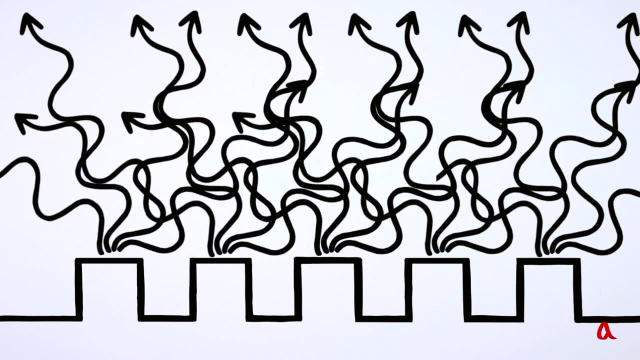 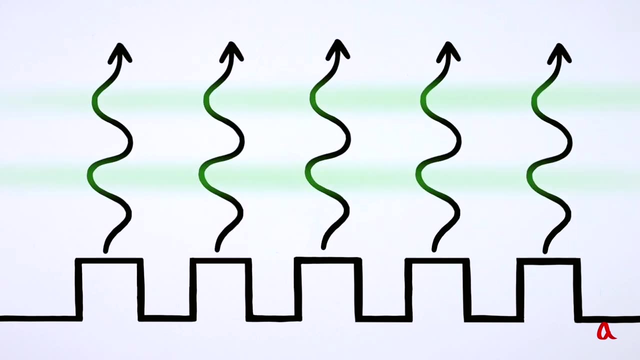 Each track of the disc is a re-radiator and the waves radiate back from it in all directions, But there are many tracks on the disc and they all emit waves simultaneously. When the waves are scattered back, their crests and troughs coincide, reinforcing each other. 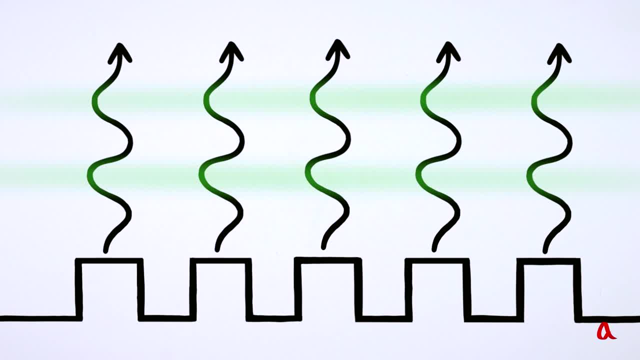 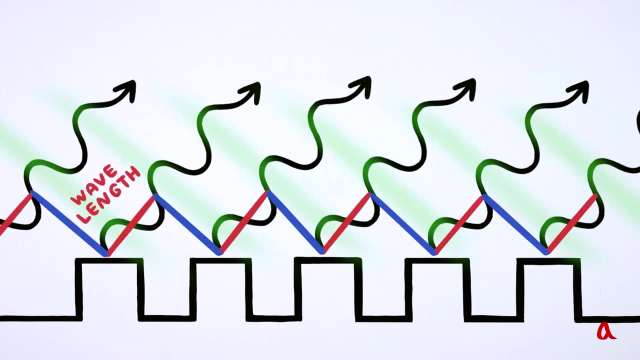 A bright spot appears on the screen in this direction, as by normal reflection. However, the crests can also coincide when the waves scatter at an angle to the disc. Here, the path difference between them is one wavelength, and in this direction bright spots will be visible too. 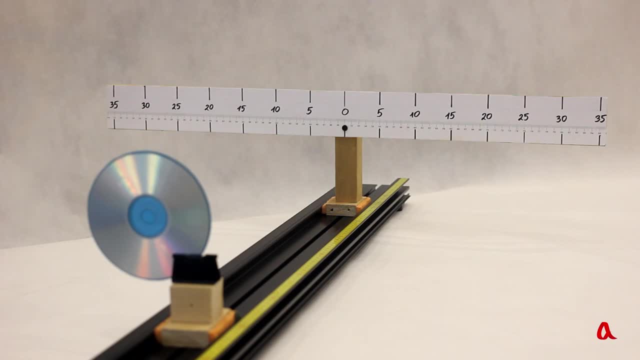 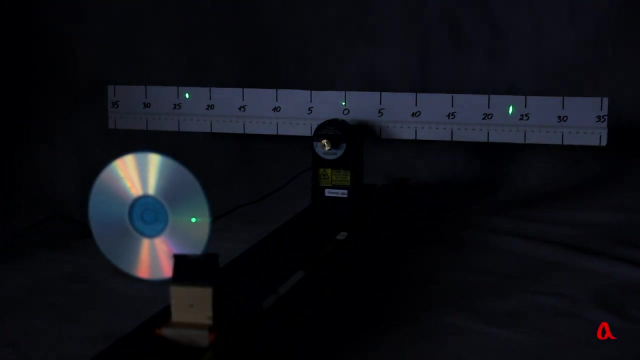 Let us install the CD onto an optical bench. We'll put a green laser in front of it. Several bright spots are visible on the screen. The central spot corresponds to a normal mirror image. The two side spots to the right and left of it have a path difference of one wavelength. 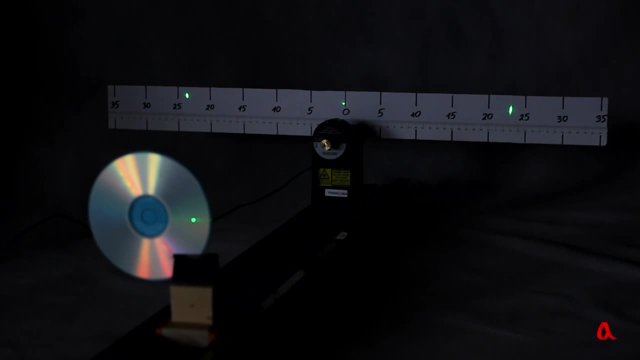 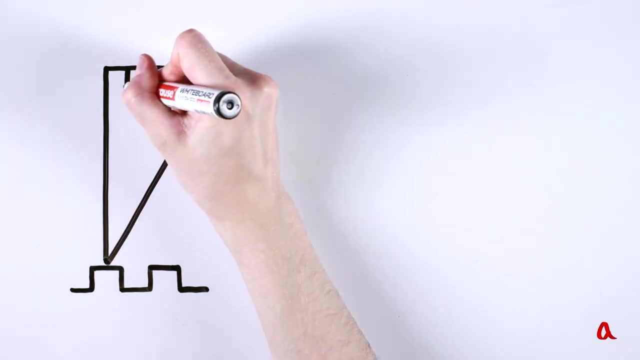 In our experiment the distance from the disc to the screen is 60 cm. The distance from the central spot to the first side spot is 23 cm. Let's reproduce the conditions of our experiment in a drawing. The legs of this right triangle are known to us.